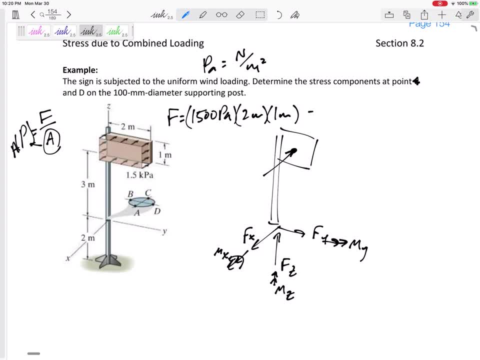 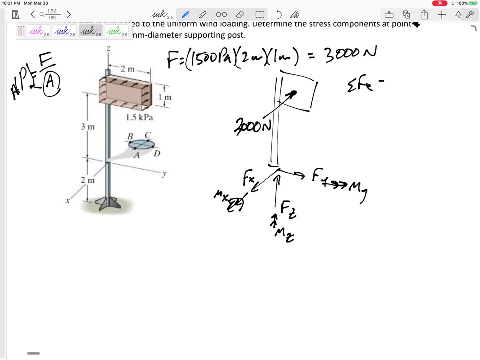 That would leave me with units. Alright, so this would be 3000 Newtons. so we can replace this one force, this pressure, with a force of 3000 Newtons, right there, Okay, so now, when I'm ready to sum the forces in x, sum the forces in y, sum the forces in z, I might have an Fx. I might have an Fx. 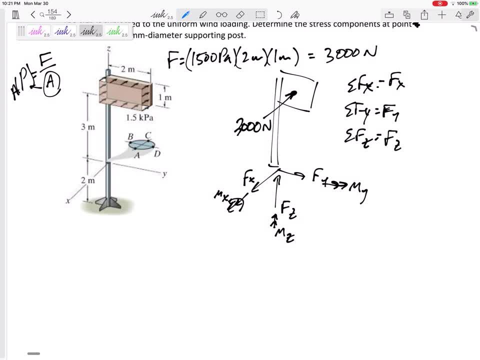 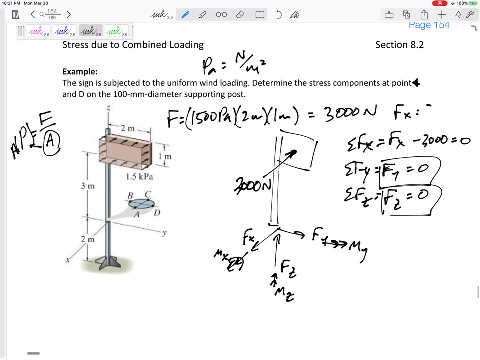 I might have an Fy, I might have an Fz, but the only thing that's really counteracting is this 3000 in the negative x. so Fz is 0,, Fy is 0, and Fx would be 3000 Newtons. right here. 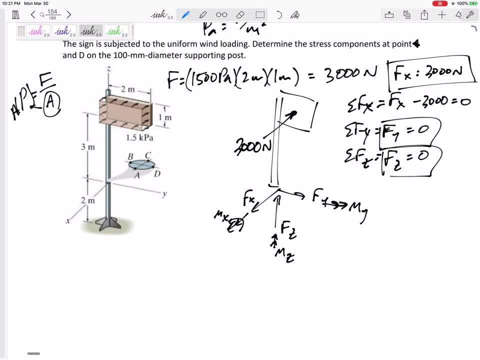 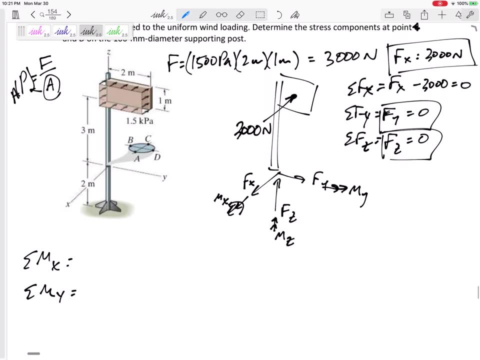 So those are the internal forces. How about the internal moments? How about the internal moments? I could sum my moments in x, sum my moments in y, sum my moments in z. I might have an internal Mx, an internal My, an internal Mz. 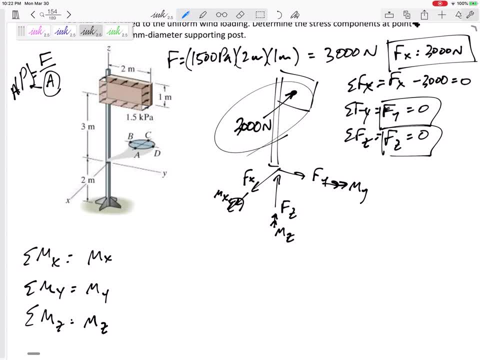 What kind of moment would this 3000 Newton force create? It might create two If it is offset from the cut in two directions, and I think it is offset in the cut in two directions. Sorry here, let's see here. 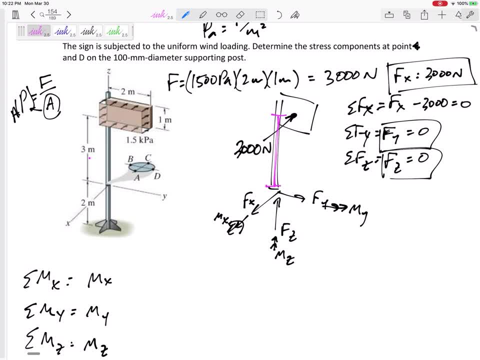 It is offset, It is. It is three meters above the cut right. It is three meters above the cut. It is also acting at the middle. Sorry, sorry, sorry. It's not three meters, not just three meters, It's three meters. sorry, to the bottom of this sign. 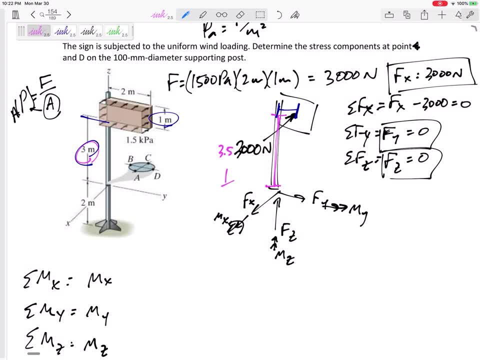 So it would be 3.5 meters to the middle right there And it would be in the middle one meter offset this way, So it kind of has two moment arms. It can create two moments. Which one do you see first? So I think the one that I see first is that it would cause rotation about this z-axis, right. 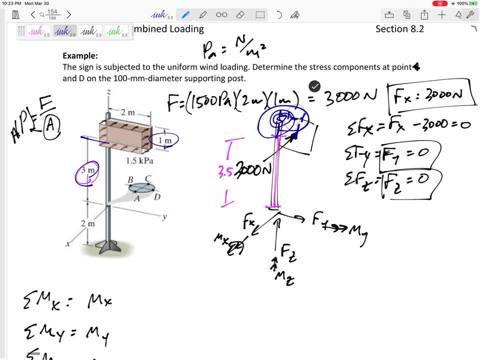 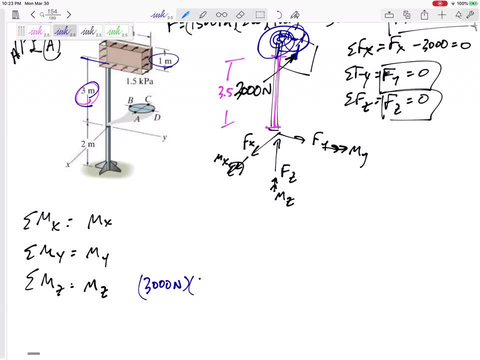 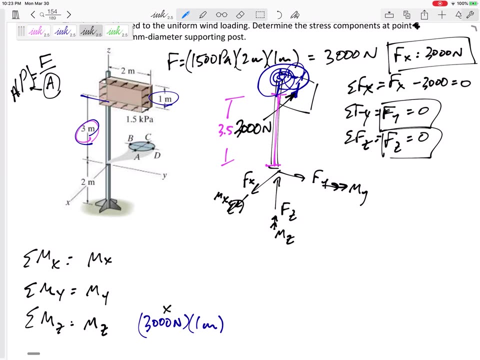 It. it's offset by one, It's over here. It would cause this twisting, this rotation in the z-axis. this 3000 Newton force With a moment arm of one would create a z rotation. Let me make sure this makes sense. This is in the x-direction. its moment arm is in the y. 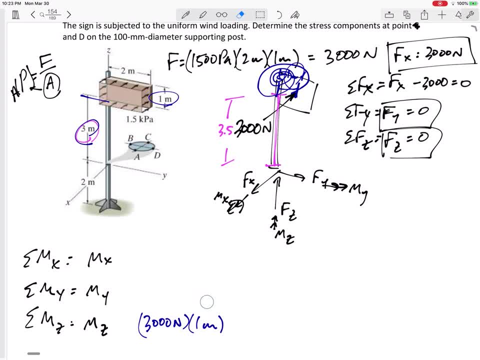 Yeah, that'd be a z moment: positive, negative. Well, would, when I curl my fingers in the rotation that it's causing, would that be positive? is my thumb pointing in positive z Using my right hand? Yes, this would be a positive Moment right here, okay. 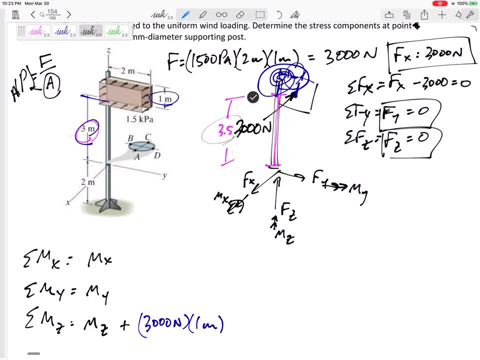 But then because it is 3.5 above the cut, it's pushing over. It's pushing over here, It's pushing, twisting about the y-axis as well: 3,000 Newtons with a moment arm, 3.5 meters. Let me make sure that makes sense. 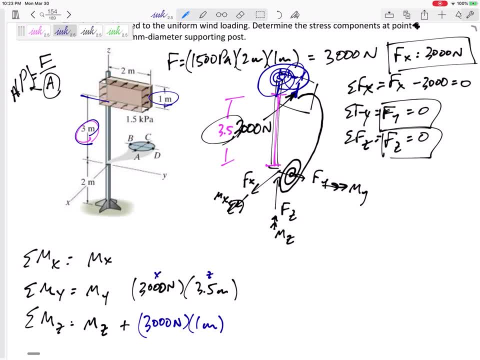 This is in the x-direction. its moment arm is in the z, Yeah x force with a z moment arm would be a y moment, positive or negative. when I curl my right hand, my four fingers in my right hand, in that Direction of the rotation, my thumb is pointing in the negative. 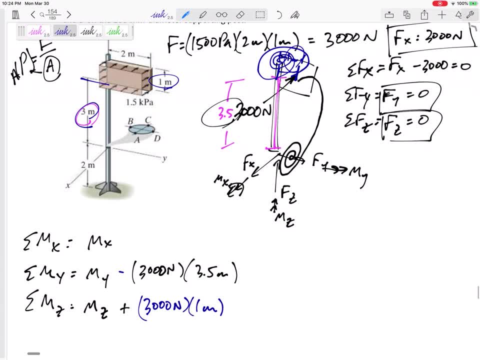 Y. my thumb is pointing in the negative y. All right, and so we'll set these equal to zero And see what we get. we've got. MX is zero, my Positive ten thousand five hundred or ten point five kilonewton meters MZ, and negative three kilonewton meters. and so there are my moments. 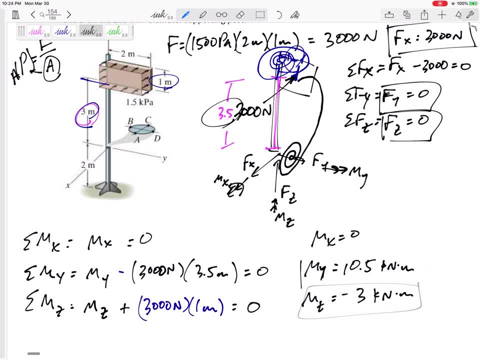 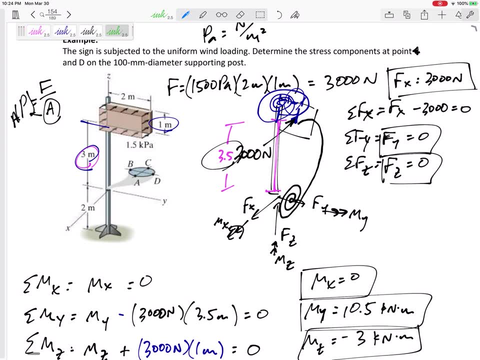 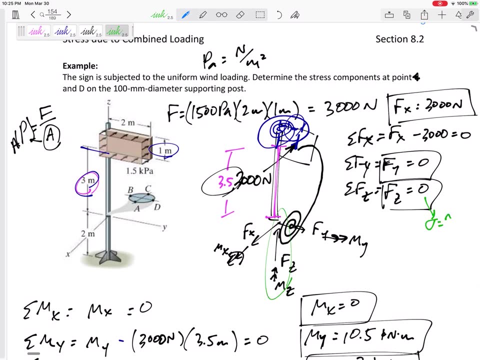 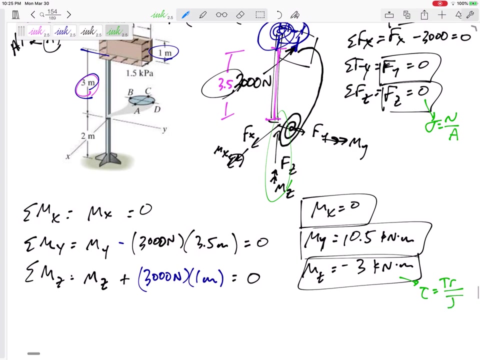 Okay, Okay now. each of these forces and moments can create a stress. I like to think of the axial one first, the one that is perpendicular in the z-direction. This could cause a normal stress of n over a. obviously it's zero right there, And this could cause a tau of TR over J. 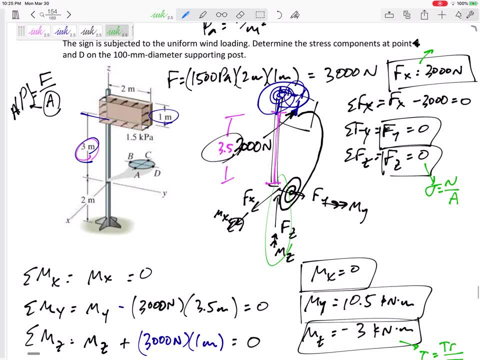 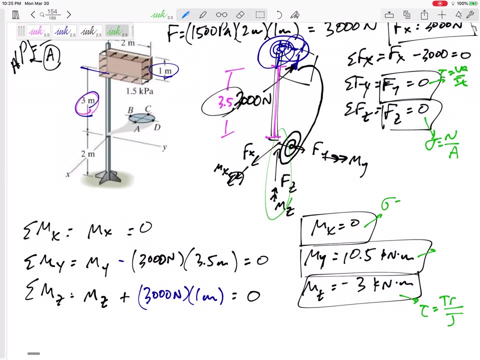 All right. and then the others, the others, these are shears That. this could cause a shear stress Vq over It. this could cause a tau Vq over It. these are bending moments. these are bending moments. Sigma, My over i, Sigma, my over I. a lot of these might be zero a. 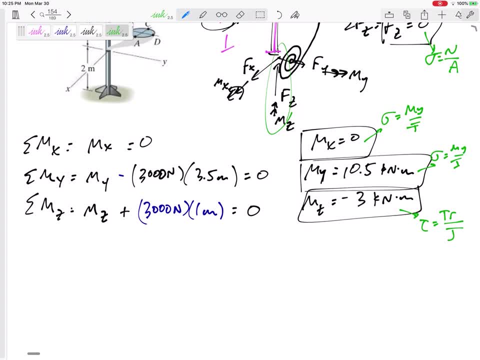 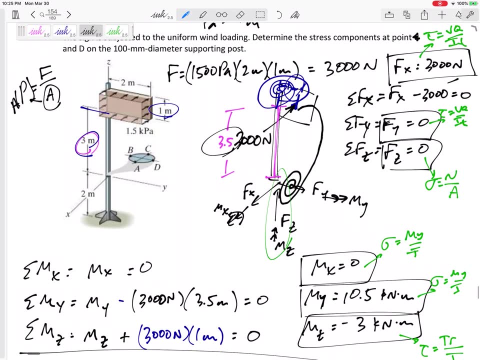 lot of these might be zero, but, um, Some of them aren't and we will calculate each of them. Okay so, Okay. so let's start with this Fx, this 3,000. right here I've got an Fx of 3,000 newtons. 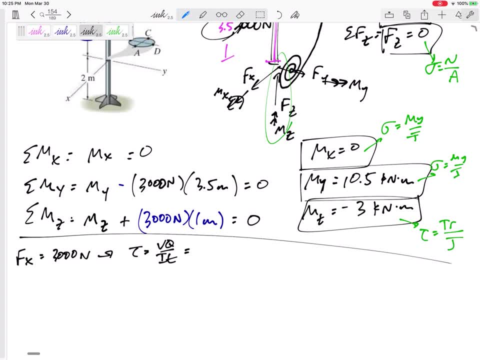 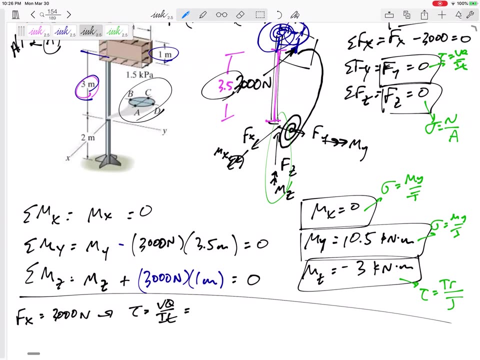 It could cause a Vq over It, a shear stress. but maybe it's zero, maybe it's not. It depends on the point that we're looking at. Let's look at point D right here. So here's my cut. I have a positive 3,000 internal force. 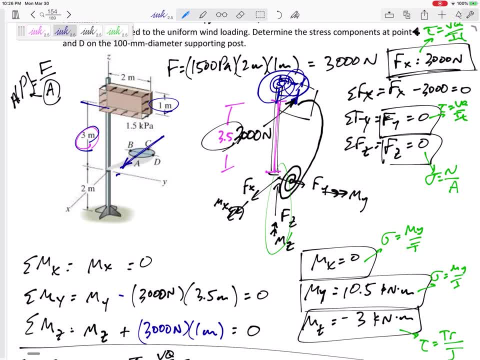 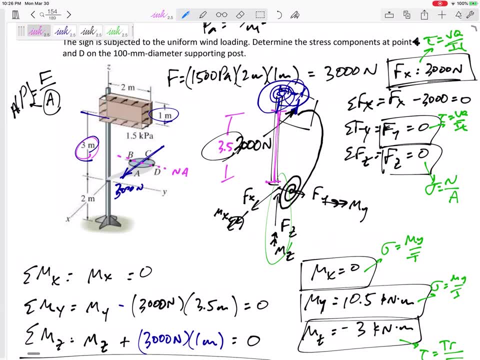 I have a force right here of 3,000 newtons. All right, my neutral axis for a V, my neutral axis would be right here And the shear stress on the neutral axis is the maximum. So yeah, point D here does have a Vq over It. 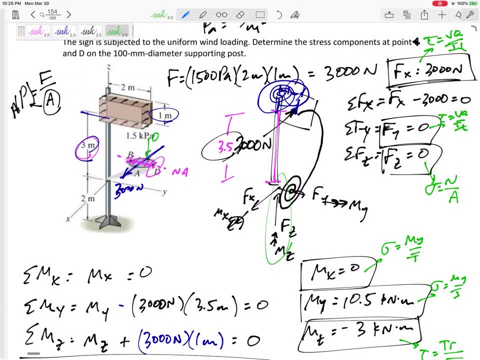 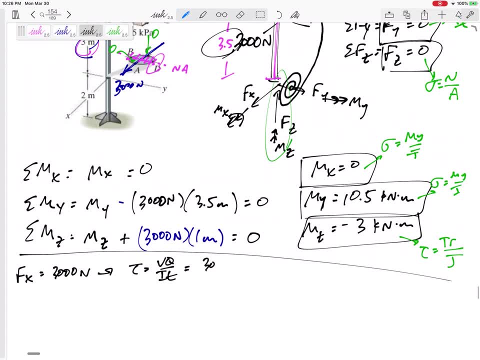 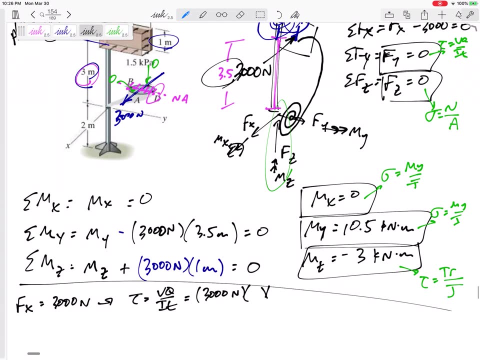 Whereas if we were looking at point C, it would be zero, Point A It would be zero, But point D does have a Vq over It. So the V would be the force: 3,000 newtons. The Q, the Q, is Y, prime, A prime. 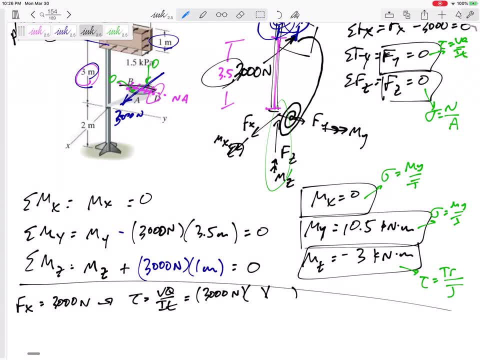 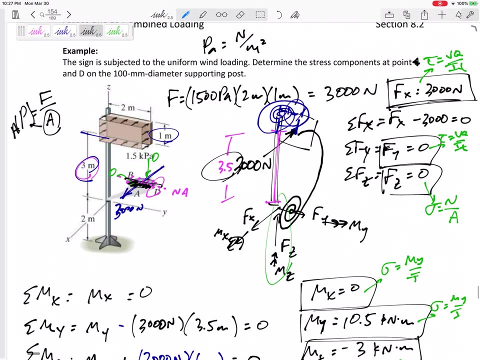 Let me come back to Y prime. But the A prime is the distance away from my point D. So this would be half of pi R squared. The R, Yeah, 100 millimeter diameter, The R would be 50 millimeters squared. 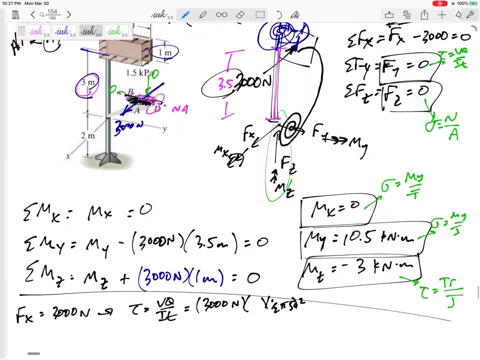 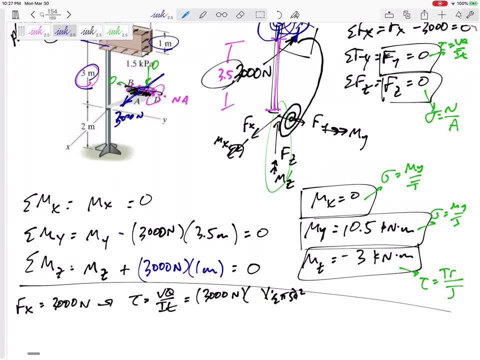 The Y prime would be the distance from the neutral axis to the centroid of that A prime. Look at your formula sheet. The centroid of a half circle is pi. by is 4R over 3 pi The Y bar prime for a half circle. 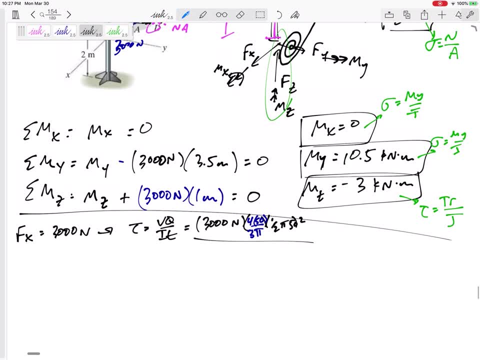 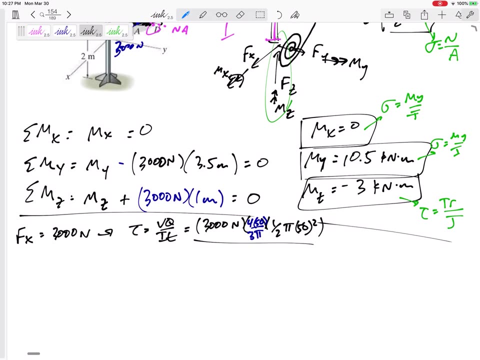 The Y bar prime for a half circle would be 4R over 3 pi. Okay, And this is the area, just an area of a half of a circle. One half pi R squared right there. All right, the I, It's just the I for the shape. 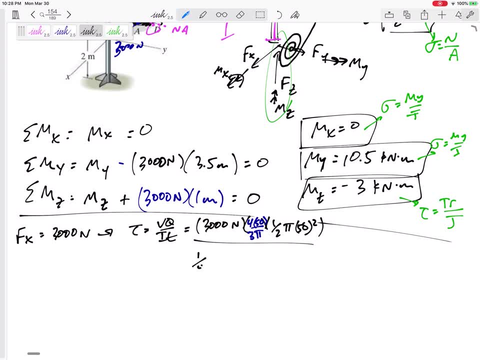 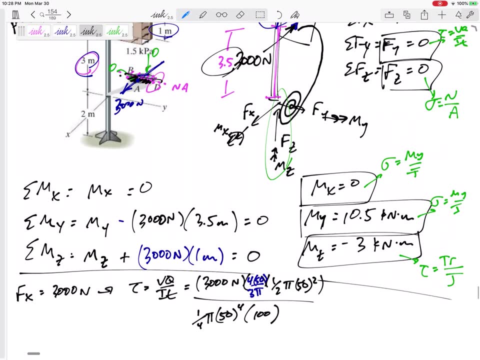 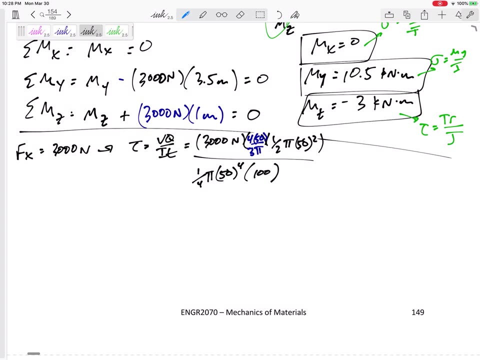 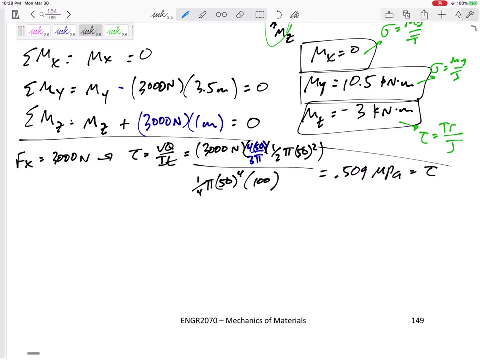 The I for the circle. The I for the circle is one-fourth pi R to the fourth And the thickness would be this thickness- This across right here- which would be the diameter: 100 millimeters. All right, so that would be 0.509 MPa is the tau. 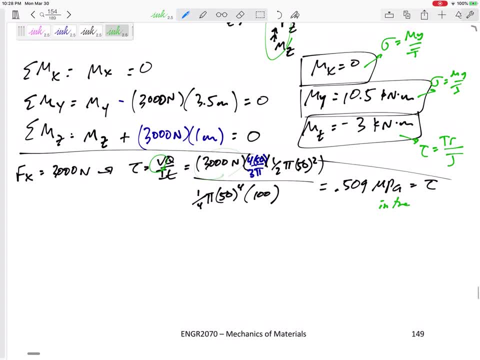 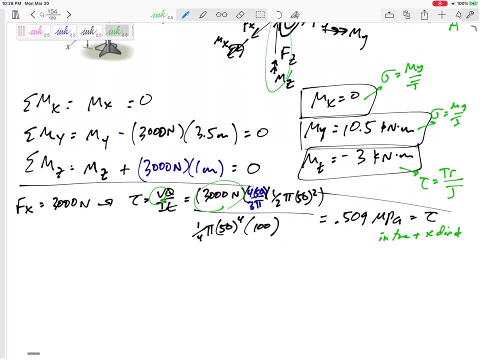 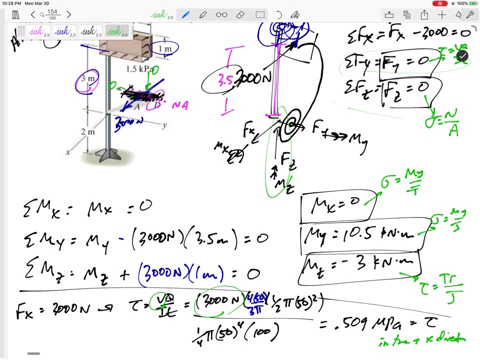 In what direction? In the- well, the direction that that V was in, The direction: the positive X direction. Positive X direction. Okay, All right, Now FYI. FYI is zero, We don't have to worry about it. 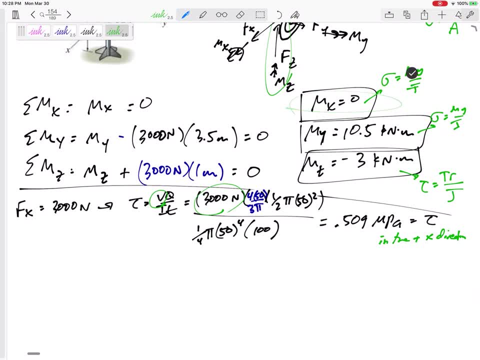 FZ is zero, Don't have to worry about that. MX is zero, Don't have to worry about that. All right, so let's go to MY. Let's go to MY MY of 10.5 kilonewton meters. 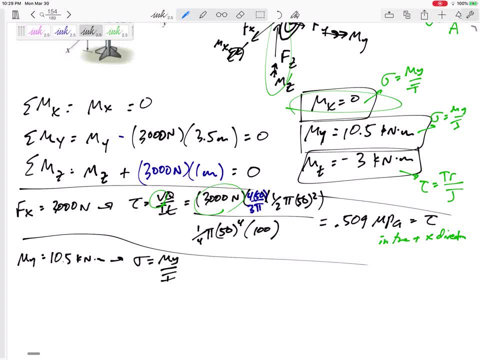 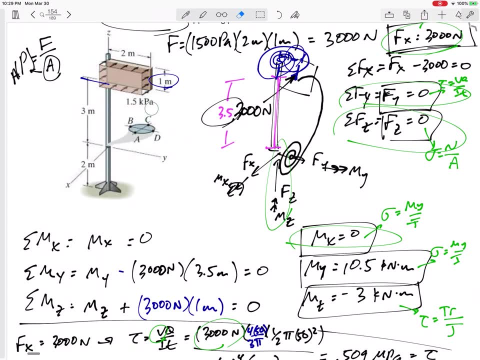 It is a bending moment. It could cause an MY over I, depending on the point. MY is bending about the Y, It's bending about the Y axis, and so the neutral axis is the Y axis. so here is my neutral axis. 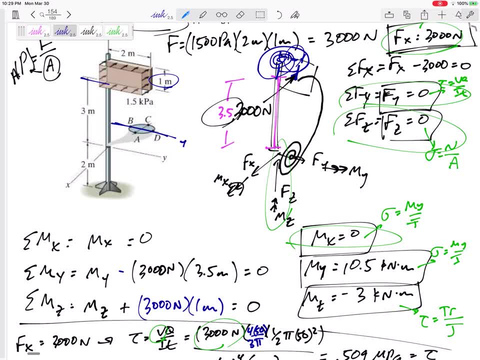 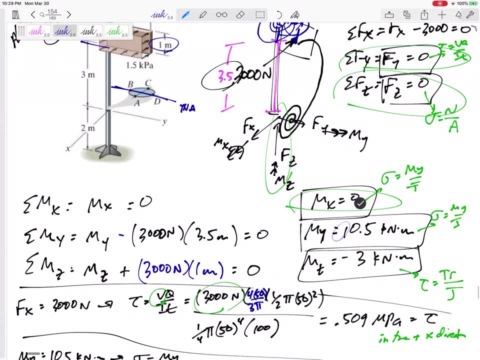 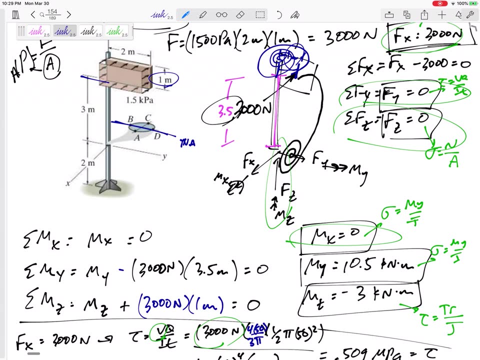 Here's the Y, my neutral axis, and it's bending about that axis. It's a positive Y moment, and so I would curl my fingers in the positive Y and there would be compression on this side. There would be compression on this side. 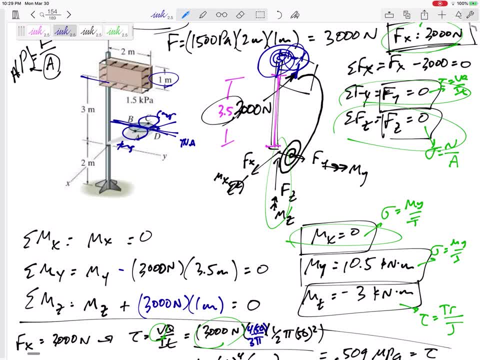 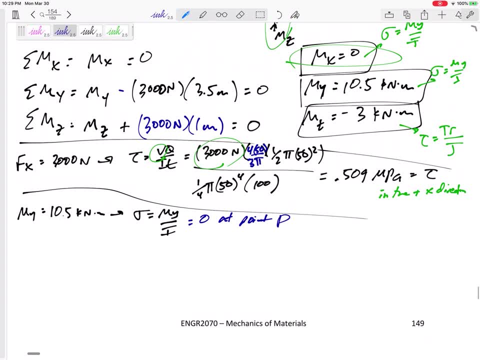 There would be tension on this side, but on the neutral axis, point D, it's going to be zero. Zero at point D. If we were looking at point C, it would be compression and we could do the MY divided by the I. 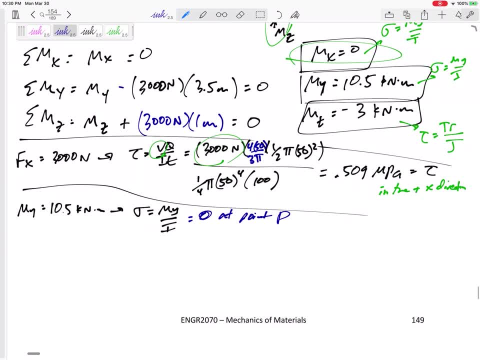 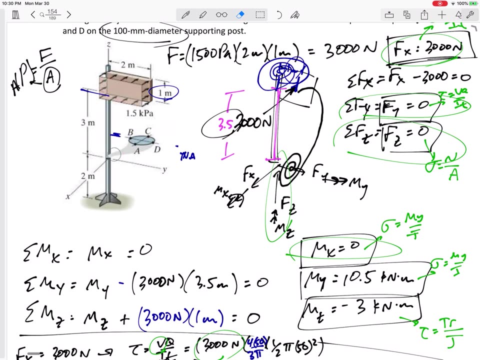 But for point D it's zero. All right, Then MZ, An MZ of negative three kilonewton meters. It could cause a T TR over J shear stress, All right. So if it twists in the negative Z direction, my thumb is not pointing positive Z. 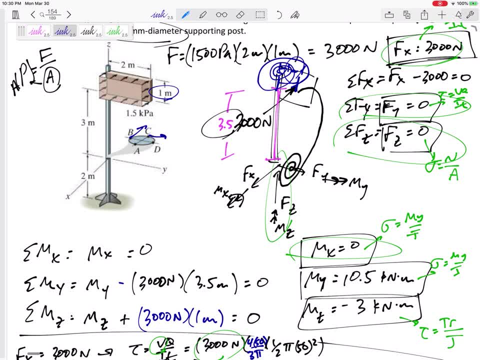 My thumb is pointing negative Z, That would kind of look like this type of stress, And so at D, it definitely has some stress and it is in this positive X direction. TR over J. Okay, so this would be a T of three. 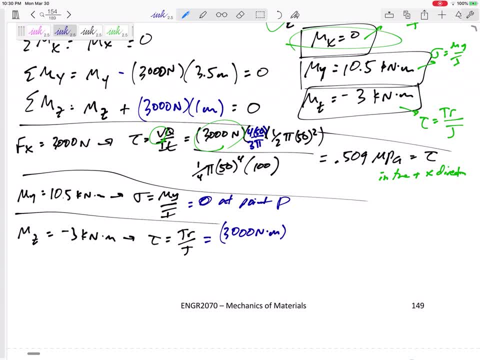 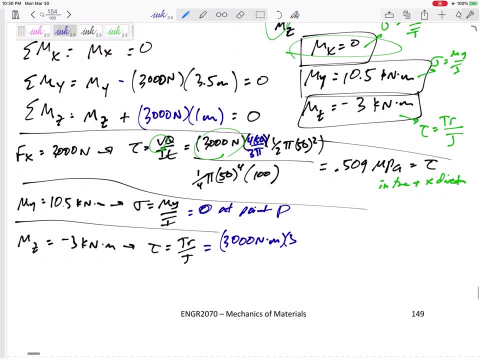 Let's do 3,000.. Newton meters Might have to change that. The R just the distance that your point is away from the center of rotation, 50 millimeters. The J pi by 2, radius to the fourth. 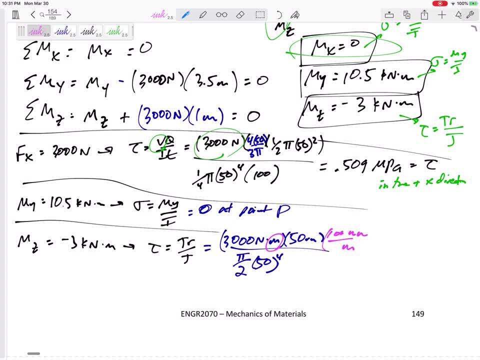 The units don't work out. I need to get rid of that meters, Change it to millimeters, So multiply this times 1,000, right there, And yes, I've got a stress of 15.. 15.3 MPa is my Tau in the positive X direction. 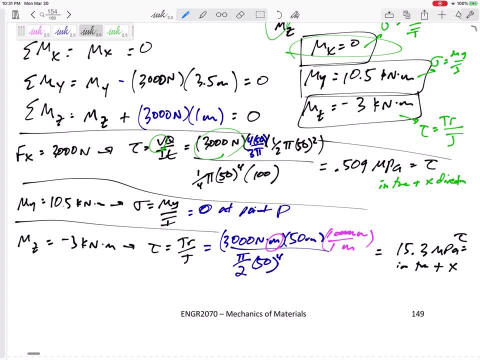 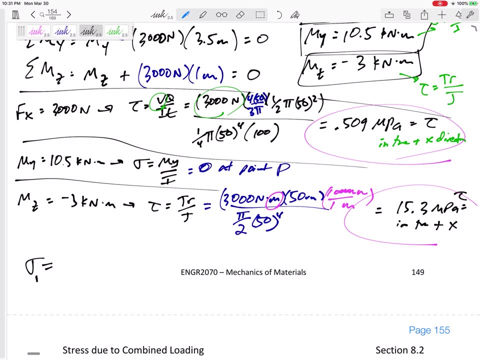 Okay, now I need to look at all those stresses and combine similar stresses in similar directions, The stresses that I've calculated. well, those are the only ones. What is the normal stress at point D? Zero, Zero. There was nothing. 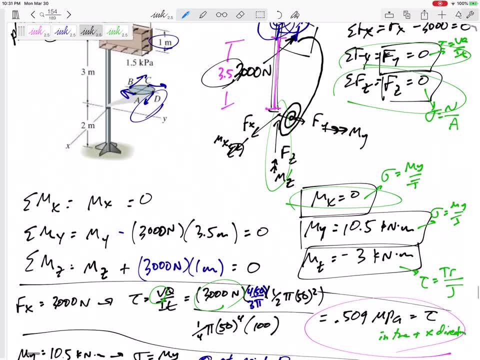 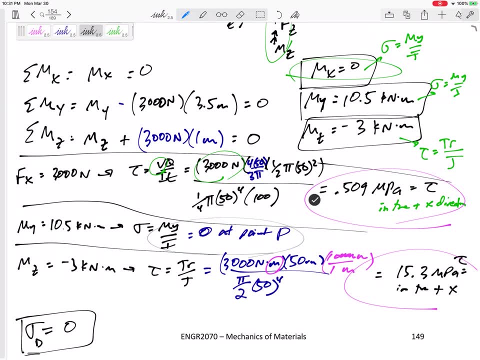 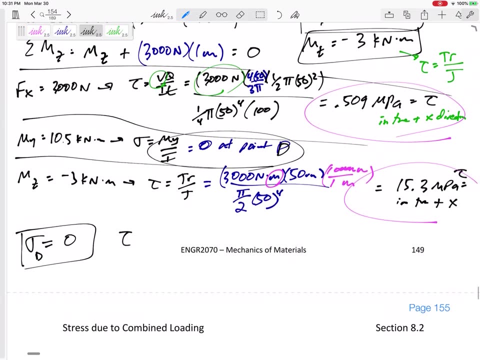 There was nothing because there was not a lot of forces, There was no FZ and there was no bending moments at point D that created any stress at point D. But there's some Tau, There's two Tau's, and both of them are in the positive X direction. 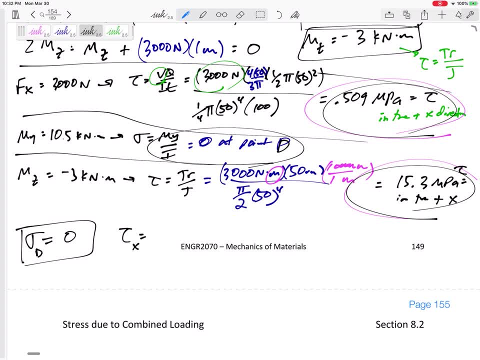 So we can add both of them up And so I'm going to call it in the. I'm going to say Tau at point D is 15.8 MPa in the positive X direction. In the positive X direction, All right. 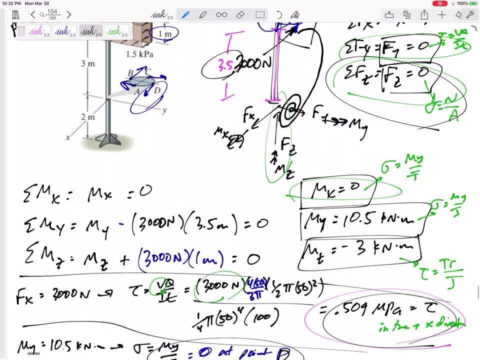 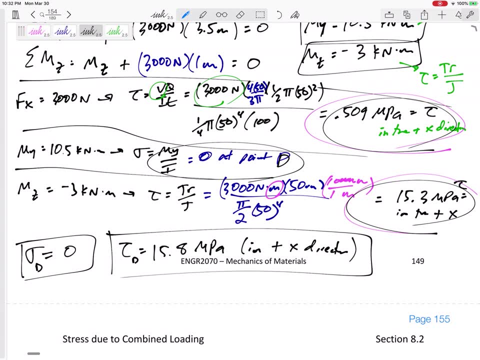 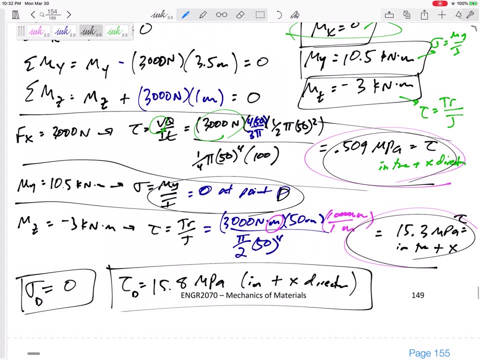 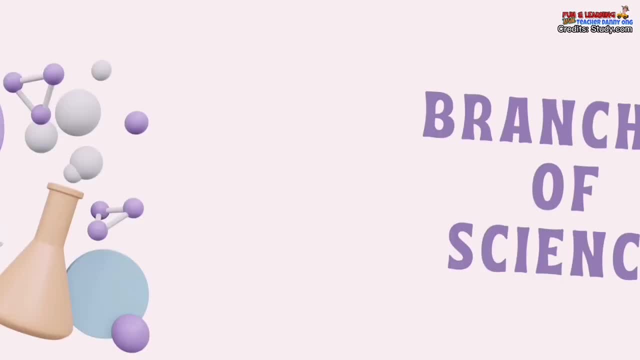 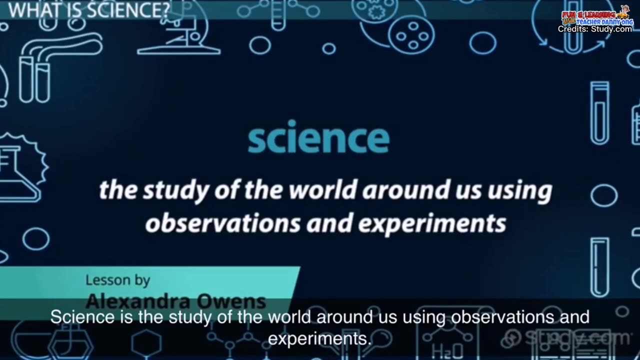 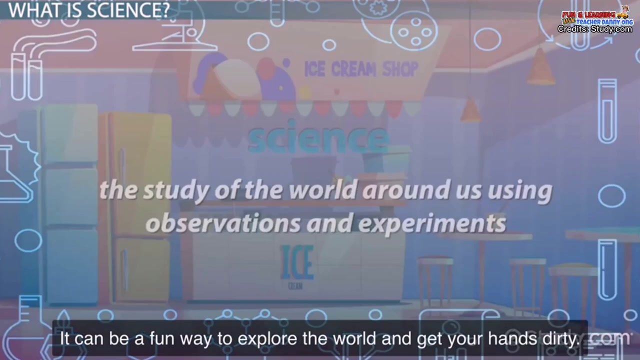 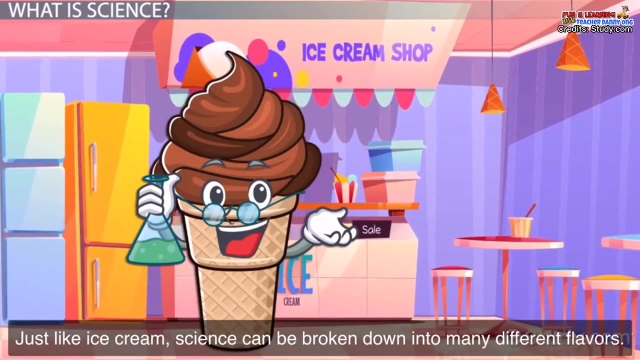 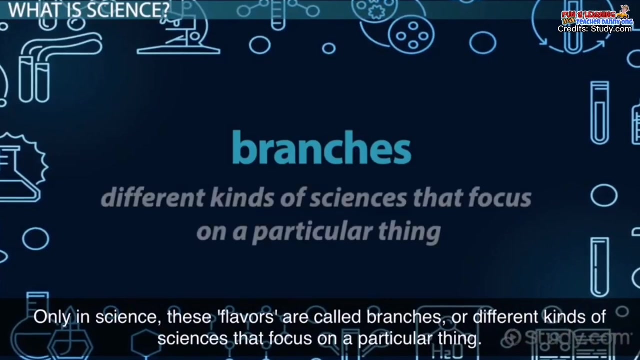 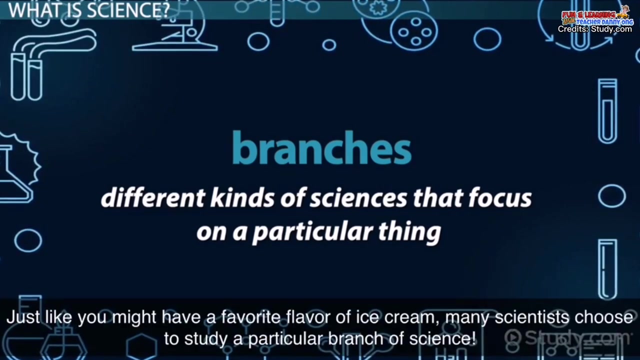 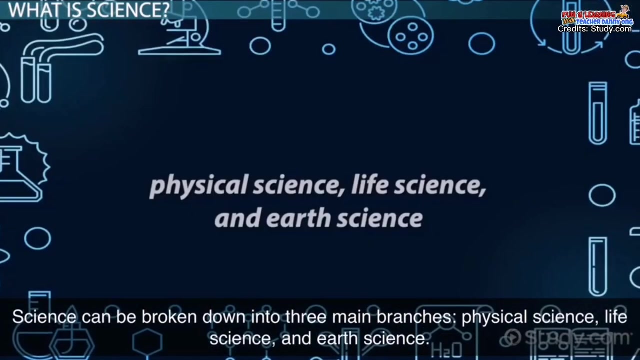 Thank you for watching branches or different kinds of science that focus on a particular thing. Just like you might have a favorite flavor of ice cream, many scientists choose to study a particular branch of science. Science can be broken down into three main branches: physical science. 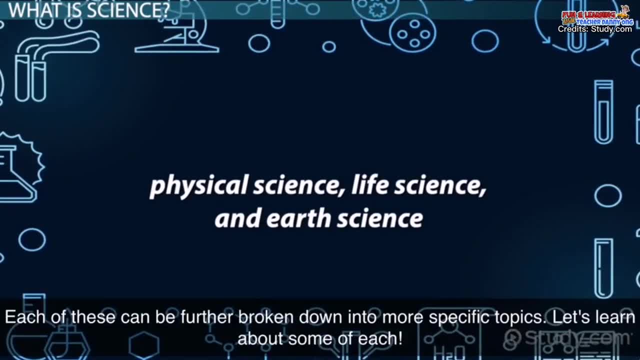 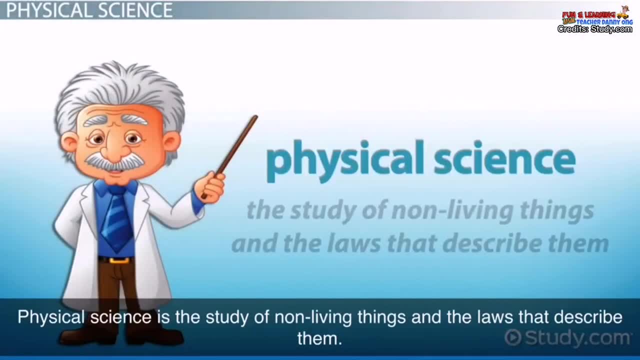 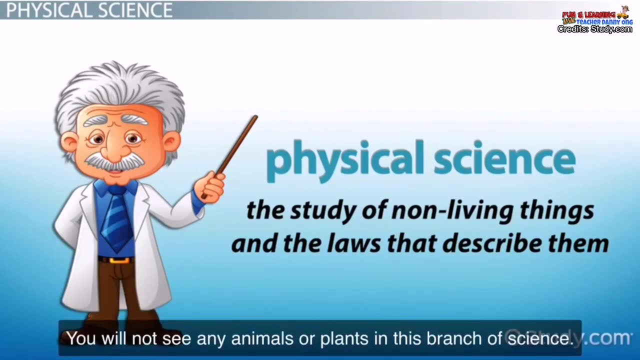 life science and earth science. Each of these can be further broken down into more specific topics. Let's learn about some of each. Physical science is the study of non-living things and the laws that describe them. You will not see any animals or plants in this. 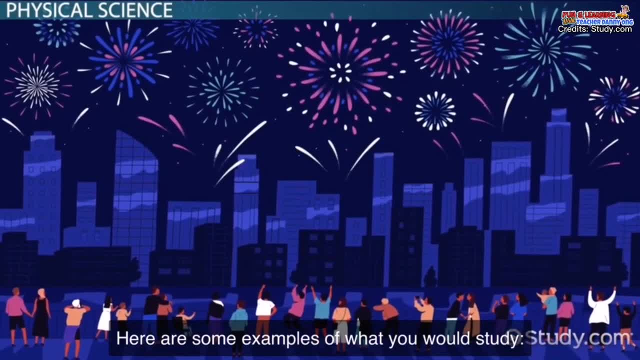 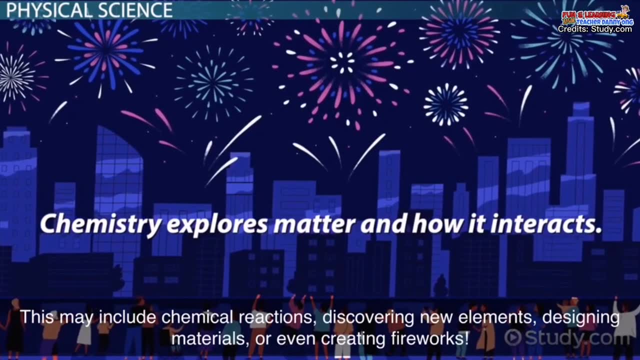 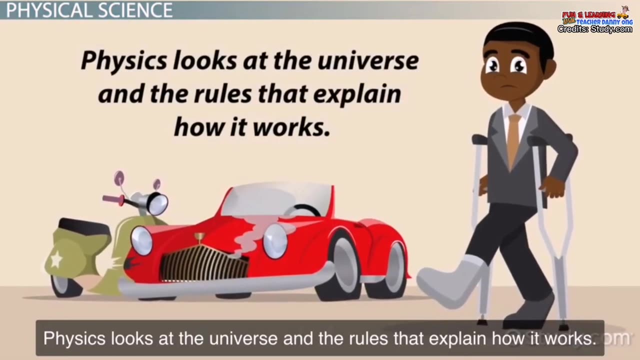 branch of science. Here are some examples of what you would study. Chemistry explores matter and how it interacts. This may include chemical reactions, discovering new elements, designing materials or even creating fireworks. Physics looks at the universe and the rules that explain how it works. In this field, you may study gravity, roller coasters, car.